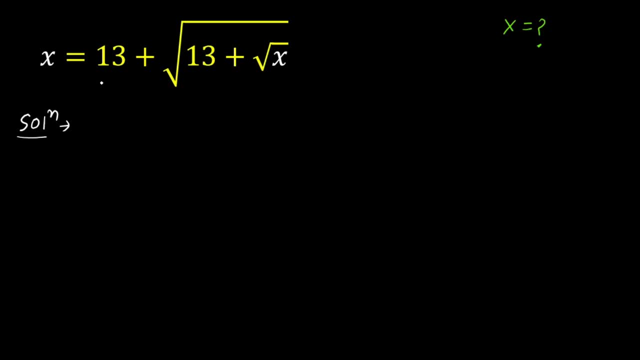 Hello students, in this video we are going to solve x is equals to 13 plus square root of 13 plus square root of x, and here we will find out the value of x. Here we will apply substitution method. If we substitute 13 plus square root of x, 13 plus square root of x. 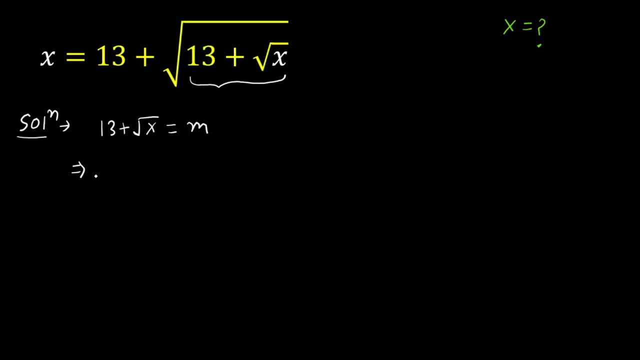 this is equals to m. This implies m minus the square root of x. this is equals to 13.. Let us consider this equation number first. Now this expression is m. this implies x is equals to 13 plus the square root of m. This implies x minus the square root of 13. 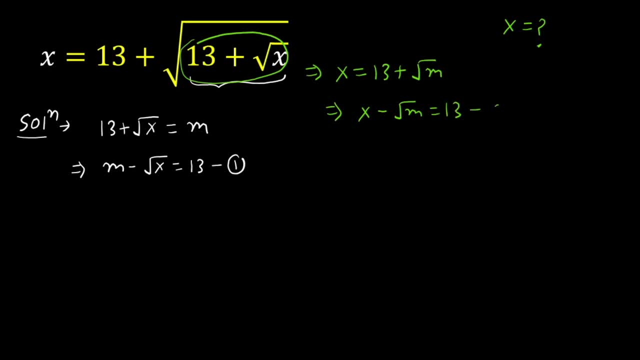 m, this is equals to 13.. Let us consider: this is equation number second. Now, if we subtract equation number second from first, then here: m minus square root of x, this is equals to 13, and x minus square root of m, this is equals to 13.. Now here, minus plus minus in left hand side, we 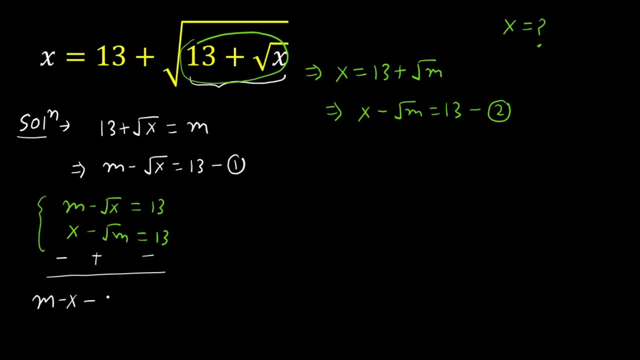 have m minus x, minus square root of x plus square root of m, and this is equals to 0.. Look carefully: m minus x- here we will apply this rule: a is equals to square root of a whole square. then this m is square root of m whole square minus x. 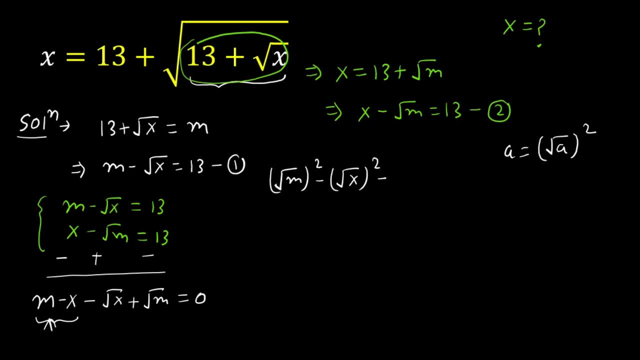 is square root of x, whole square minus square root of x plus square root of m, and this is equals to 0.. Here look carefully these two terms. if we apply difference between two squares, a square minus b square, this is equals to sum of a plus b times difference between a minus b. Here we can: 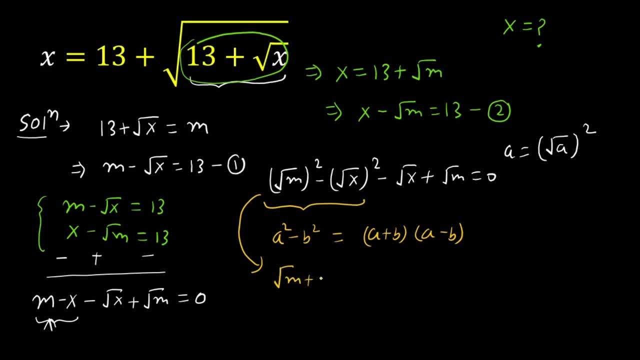 say, square root of m plus square root of x is multiplied by square root of m minus square root of x, and here plus square root of m minus square root of x, and this is equals to 0.. Now, if we take common square root of m minus square root of x, square root of m minus square root of x. 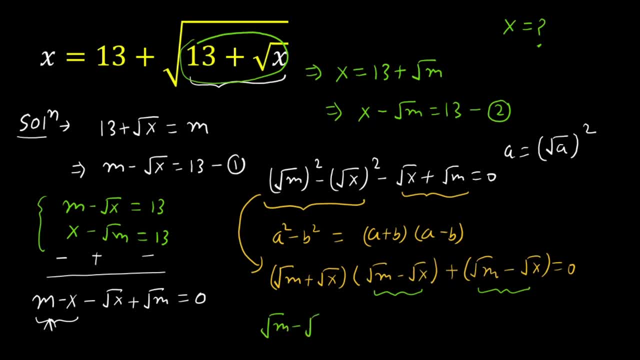 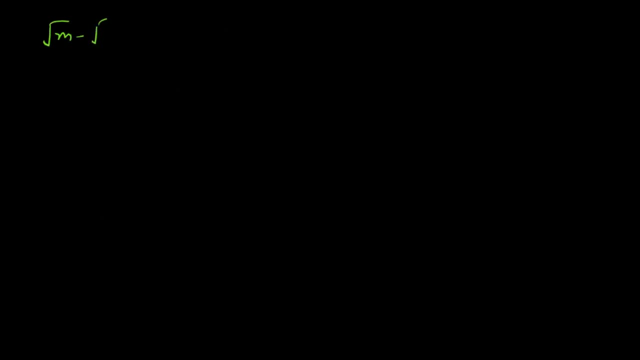 is common, then square root of m plus square root of x plus 1, and this is equals to 0.. Then square root of m minus square root, x is multiplied by square yard- ok, please- by x plus 1, and this is equals to 0.. Here we will apply this rule. if this is equal to 0 or l, here we will apply this rule. 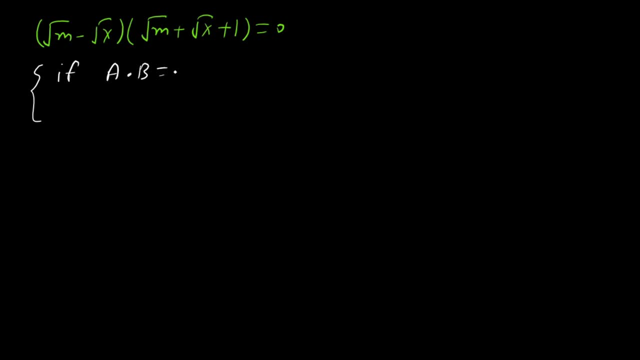 A times B, this is equals to 0. this implies A is equals to 0 or B is equals to 0. Then here, square root of M minus square root of X, this is equals to 0. square root of M plus square root of X. 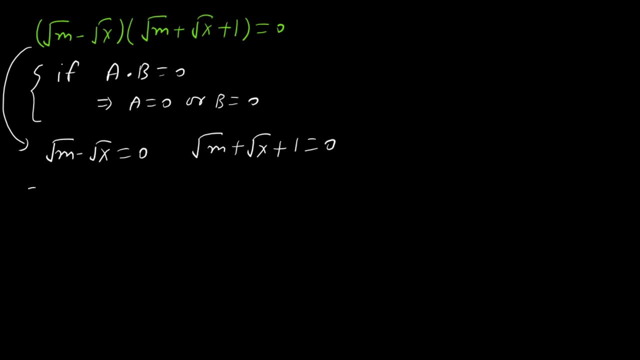 plus 1, this is equals to 0.. This implies square root of M. this is equals to square root of x, and if we take square both side, then we can say m is equals to x Here. this is case. first, Look carefully these terms. This implies square root. 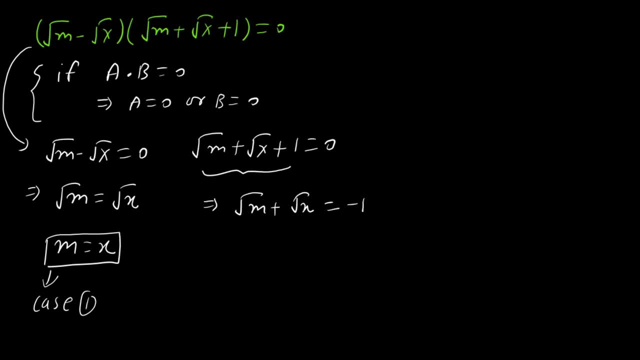 of m plus square root of x, this is equals to minus 1.. Here, left hand side, square root of m is positive and square root of x is positive. It means sum of two positive number is always positive. Left hand side is positive and right hand side is negative. So that's why this case. 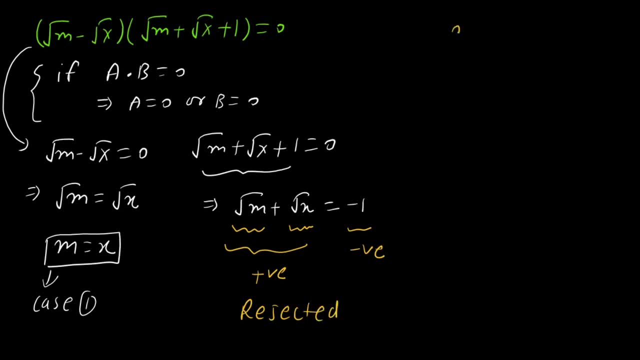 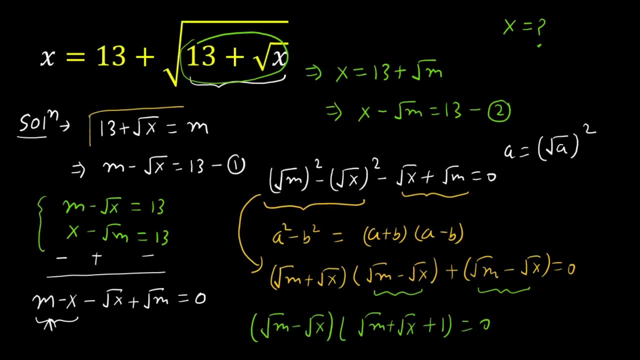 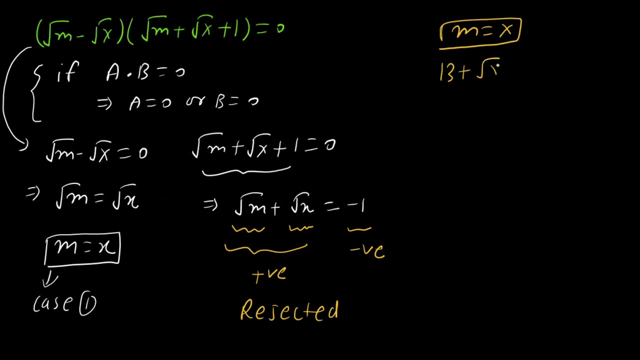 is rejected. Here m is equals to x, and we know that 13 plus square root of x, this is equals to m, 13 plus square root of x. this is equals to m, 13 plus square root of x, and this is equals to this. m is replaced by x because here m and x both. 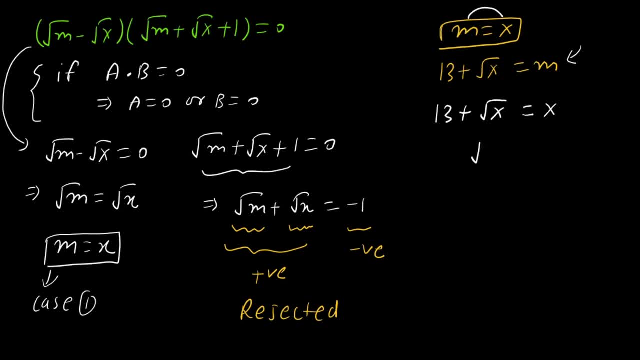 are equal, Then here x, Now square root of x. this is equals to x minus 13, and here in left hand side we have square root. So that's why if we take square both side, then in left hand side this square is cancelled out by this square root. Then here m is equal to m. 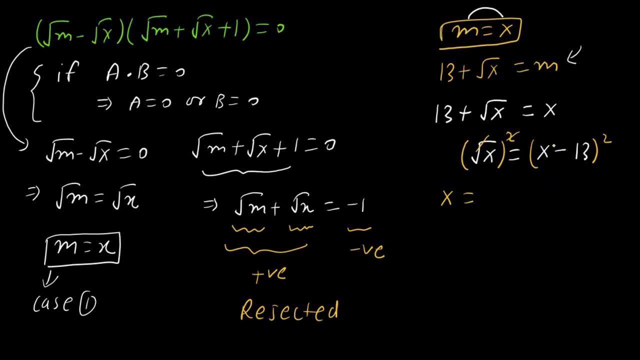 x is equals to, and in right hand side we will apply a minus b whole square. We know that a minus b whole square is a square plus b square minus 2 times ab. Then here x square plus 13 square, that is 169 minus 2 times 13 times x. Then x is equals to x square plus 169 minus 26. 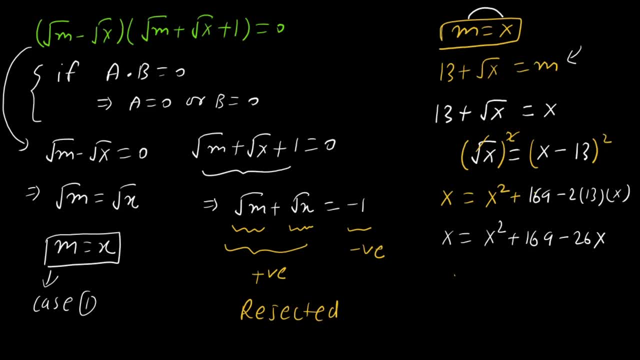 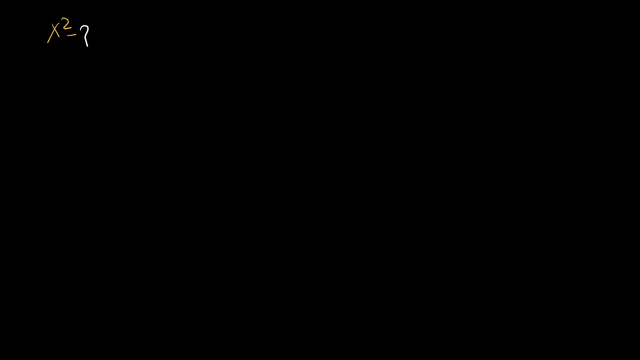 times x. Now, if we take all the expression in same side, then x square minus 27 x plus 169, this is equals to 0.. This is quadratic equation: x square minus 27 times x plus 169, this is equals to 0.. 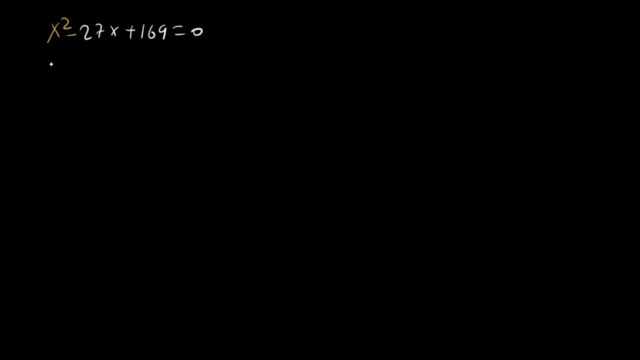 Here we will apply quadratic formula and then find out the value of x. We know that quadratic formula is: x is equals to minus b plus 169.. Then here, x square minus 27 times x plus 169. this is equals to minus b plus minus square root of b square minus 4ac divided by 2 times a And 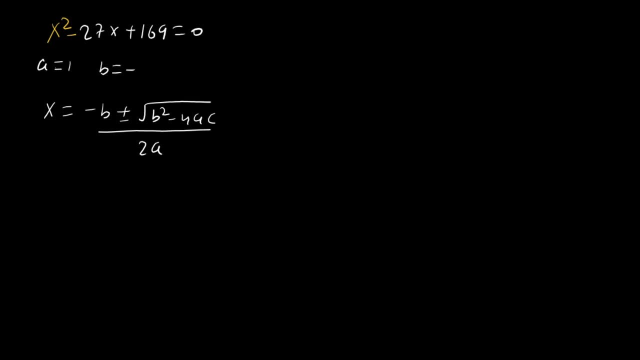 here value of a is 1 and value of b is minus 27 and value of c is 169.. Here x is equals to minus, b is replaced by minus 27 plus minus square root of, and this b is replaced by minus 27, whole square minus 4 times value of a is 1 and value of c is 169.. Then here x is equals. 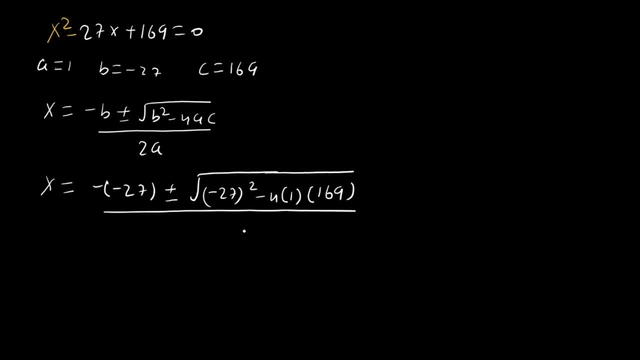 to minus b is replaced by minus b plus minus square root of minus 27, whole square that is 169. and divided by 2 times a value of a is 1.. Then x is equals to minus b. is multiplied by this minus 27, then we get 27 plus minus square root of minus 27. whole square that: 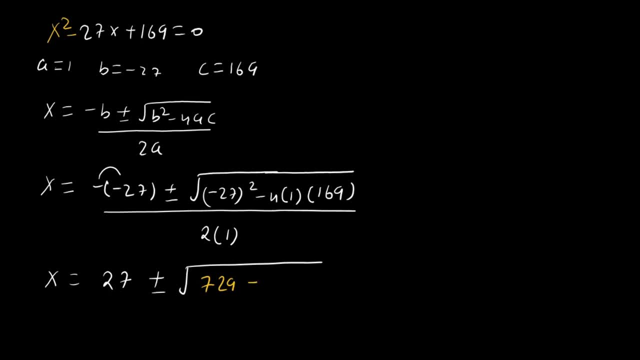 is 729 minus 4 is multiplied by 169, then we get 676 and divided by 2.. Then x is equals to 27 plus minus square root of 729 minus 676. then we get 53 and divided by 2.. Here. 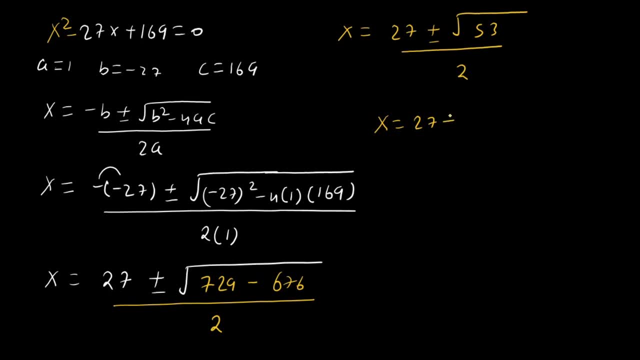 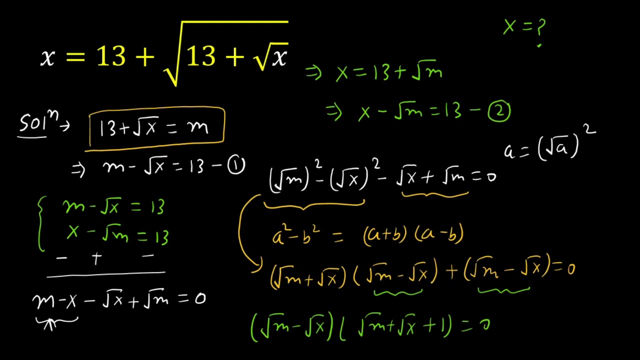 we have two possible values: of x is equals to 27 plus square root of 53 divided by 2, and second value of x is: x is equals to 27 minus square root of 53 divided by 2.. But students look carefully. the given equation, The given equation is: 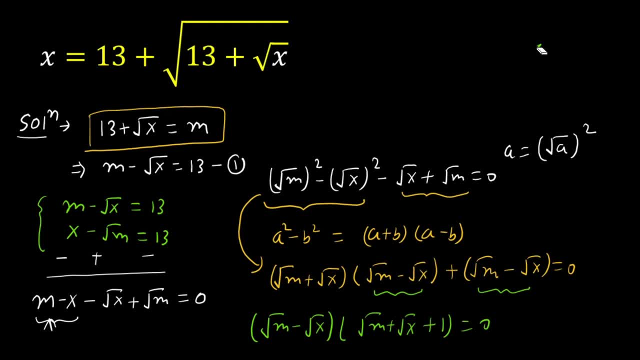 x is equals to 13 plus square root of 13 plus square root of x. This equation is same as square root of 13 plus square root of x. this is equals to x minus 13.. Look carefully: left hand side. Left hand side is always positive and this left hand side is cannot be 0.. If 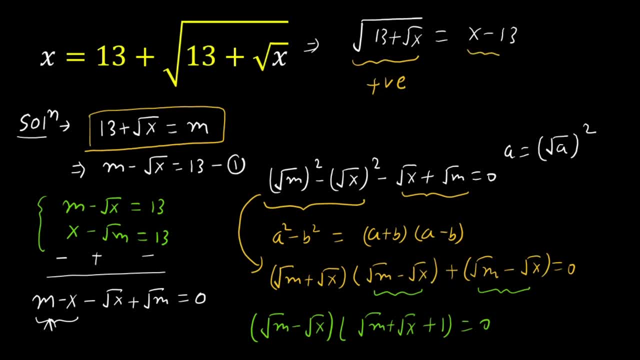 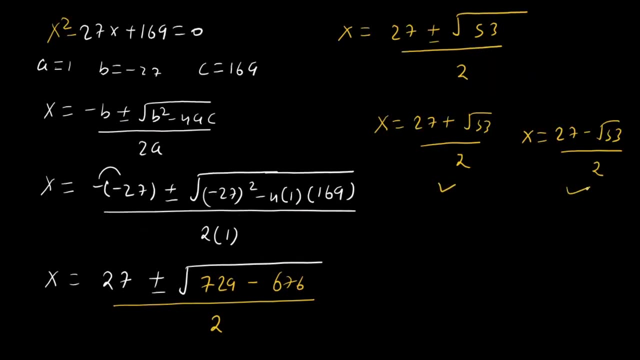 left hand side is positive, then x minus 13 should be positive. We can say x minus 13 should be positive, then here x is greater than 13.. Then look carefully these two solutions. This solution is less than 13.. So that's why this solution is rejected. 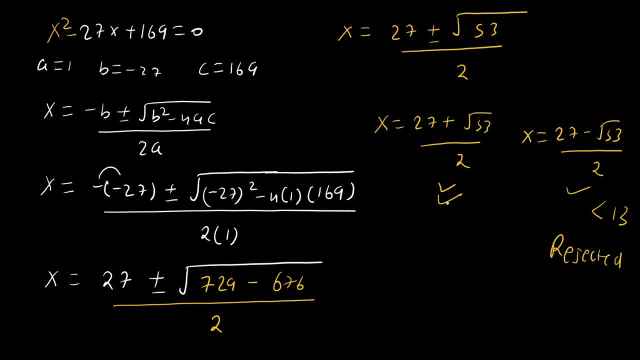 and this solution is accepted. So here, value of x is 27 plus square root of 53, divided by 2.. This is our final answer. Students, if you like my video, then please like and subscribe. Thank you. Please, then please subscribe my channel and thank you.